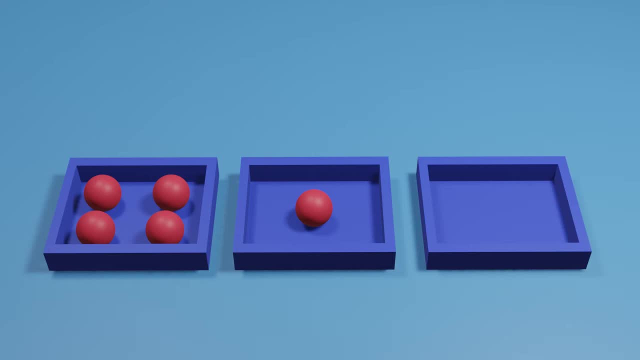 one in another and zero in the last box. We will call this arrangement 4-1-0.. Another arrangement we can do is three in one box, two in another and zero in the last box. We will call this arrangement 3-2-0.. Another arrangement we can do is three in one box. 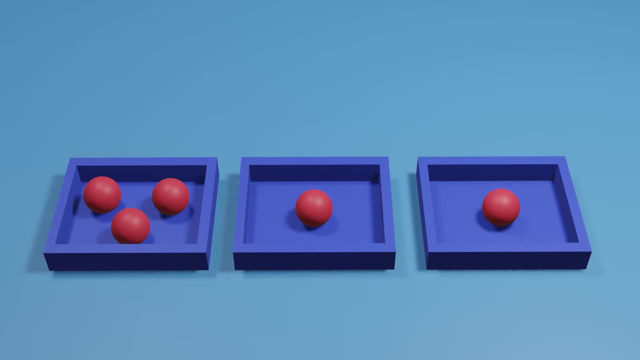 one in another and one in the last box. We will call this arrangement 3-1-1.. Another arrangement we can do is 2 in one box, 2 in another and 1 in the last box. We will call this arrangement 2-2-1.. 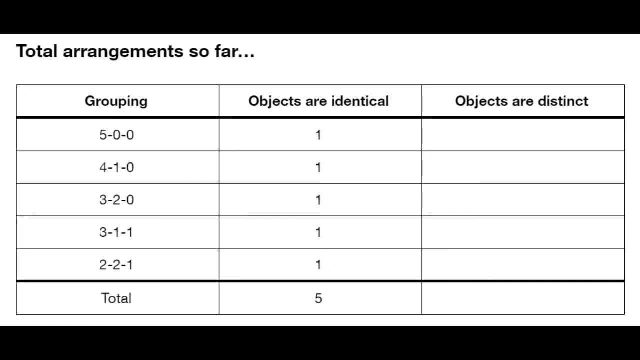 That lists all the arrangements for 5 identical objects among 3 identical boxes. This is one way to break the problem into smaller pieces, To solve the original problem of finding the number of ways to arrange 5 distinct objects among 3 identical boxes. 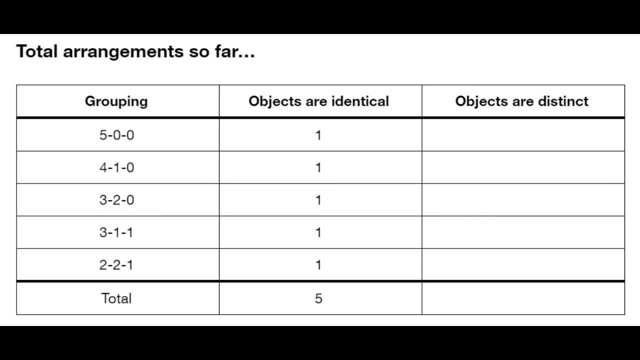 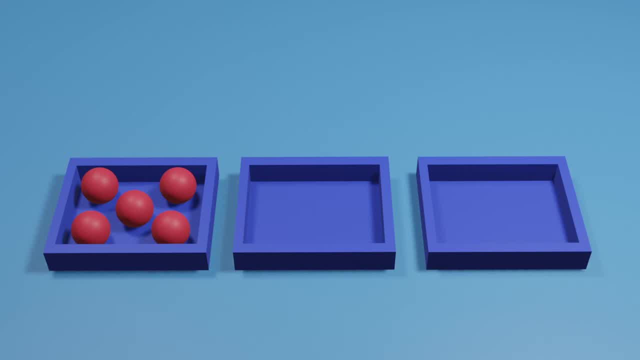 we can think what happens to each of the above arrangements when we make the objects distinct from each other. For the first arrangement- 5-0-0,, when we make the objects distinct, there is still only one arrangement. For the second arrangement- 4-1-0,, when we make the objects distinct, there are 5 ways to choose the one object that is alone. 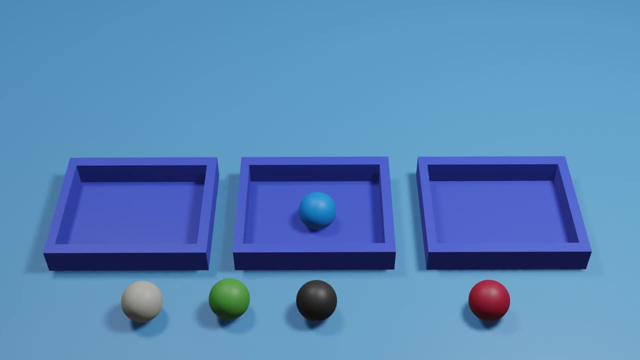 Every time you select one, the other 4 objects that are not chosen are put into another box. So there are 5 ways to choose the one object that is alone. For the third arrangement- 3-2-0,, when we make the objects distinct, there are 5 ways to choose the one object that is alone. 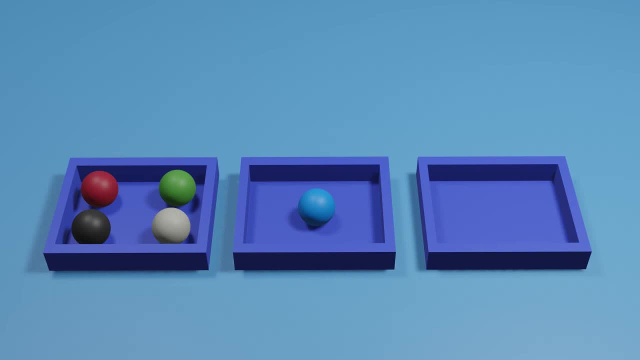 Every time you select one, the other 2 objects that are not chosen are put into another box. So there are 5 ways to choose the one object that is alone. For the third arrangement- 3-2-0,, when we make the objects distinct, there are 5 ways to choose the one object that is alone. 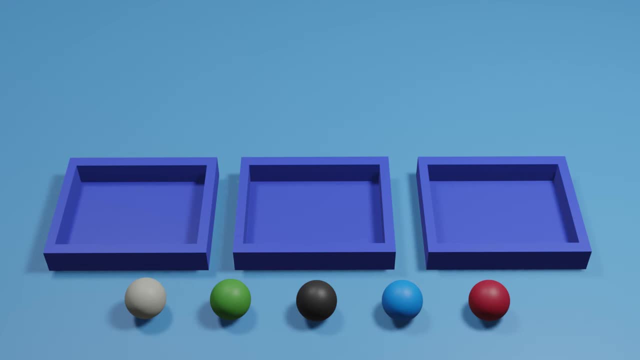 So there are 5 ways to choose the one object that is alone. Every time you select one, the other 2 objects that are not chosen are put into another box. So there are 5 ways to choose the one object that is alone. 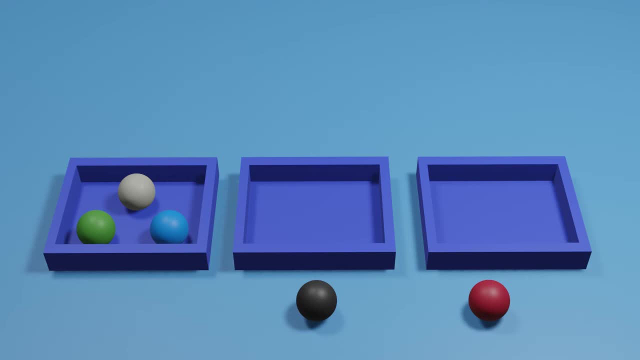 Every time you select one, the other 2 objects that are not chosen are put into another box. So there are 5 ways to choose the one object that is alone. Every time you select one, the other 2 objects that are not chosen are put into another box. 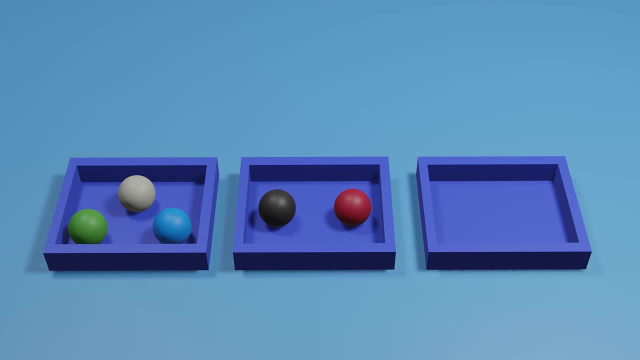 ways we can rearrange the distinct objects in this arrangement 3-2-0.. For the fourth arrangement, 3-1-1,, when we make the objects distinct, there are ten ways to choose three out of five objects. Every time you select three, the other two objects are put into one box each.